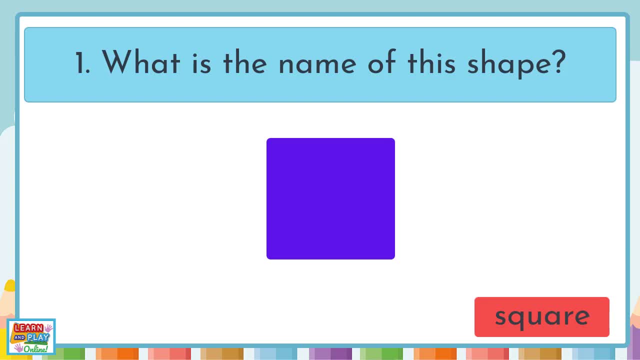 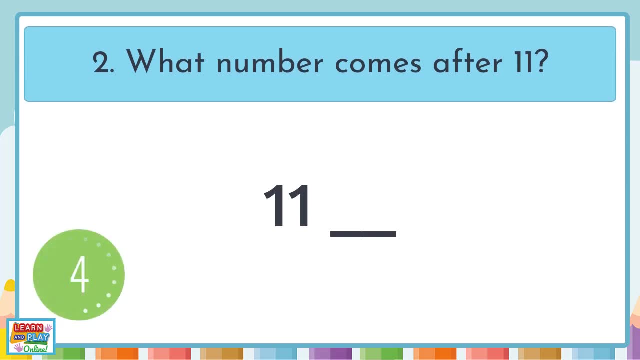 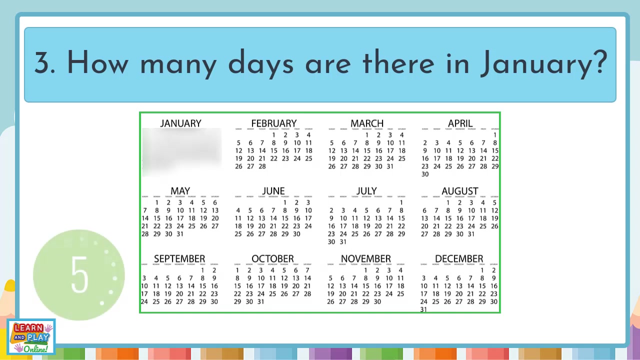 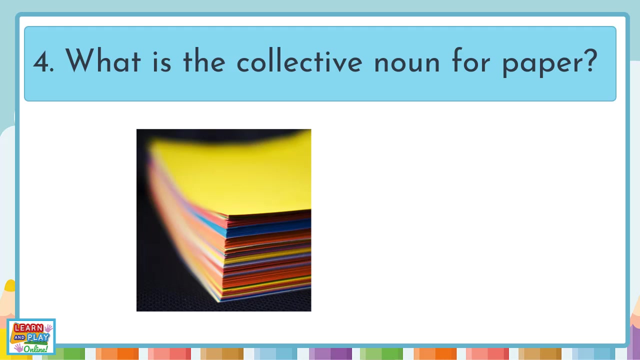 It's a square? Question 2.. What number comes after 11? 12, Question 3.. How many days are there in January? 12 days, 31, Question 4.. What is the collective noun for paper? A bunch of paper, a pack of paper or a ream of paper? 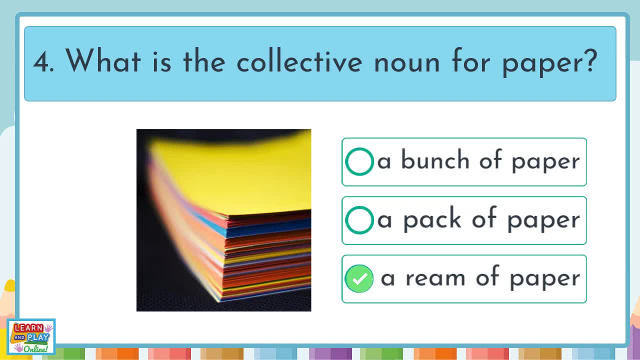 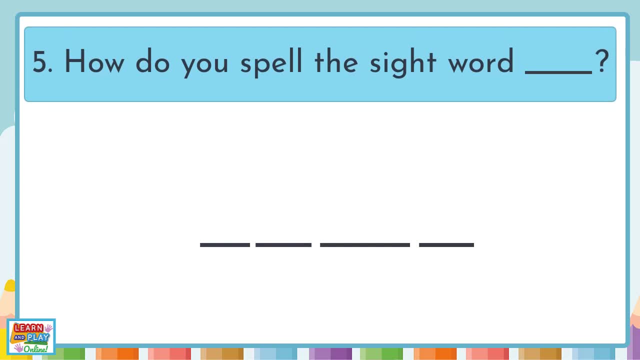 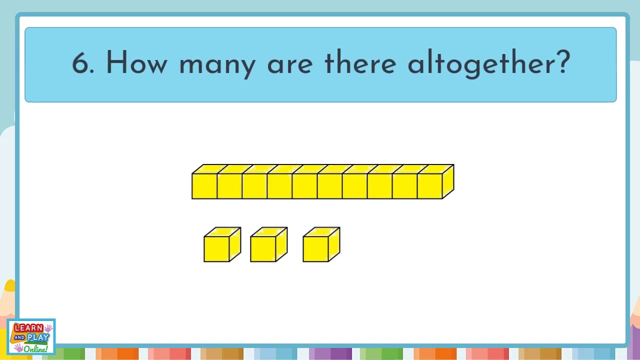 A ream of paper. Question 5.. How do you spell the sight word come C-O-M-E? Question 6. How many are there altogether? 13? Question 7.. Who does Little Red Riding Hood go to visit in the fairy tale? 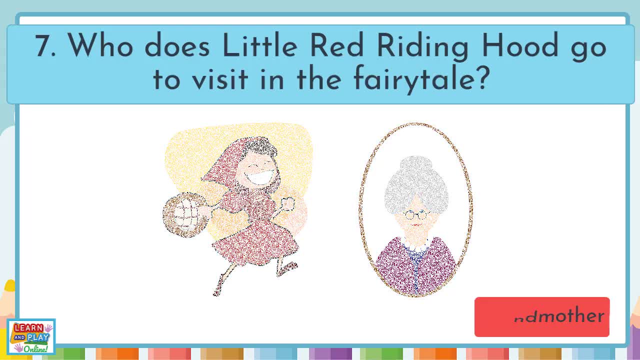 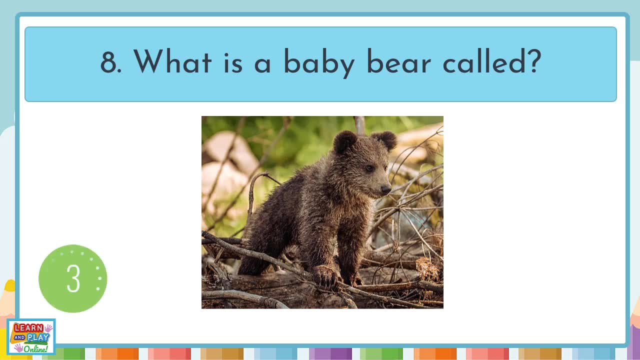 Her grandmother, Question 8.. What is a baby bear called A cub? A cub, A cub, Question 9.. Is the number 7 an odd or even number? A cub, Question 10.. Which word rhymes with pet? 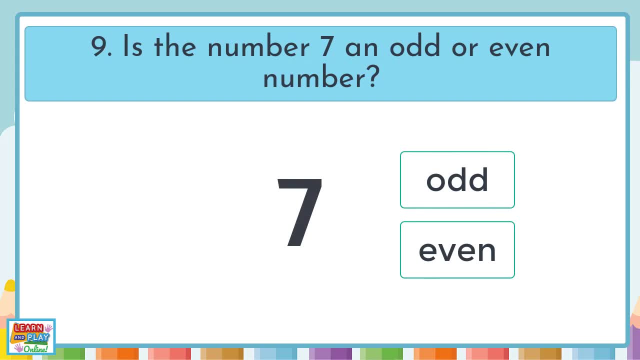 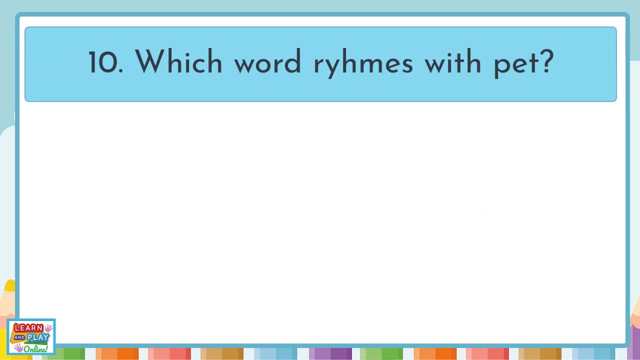 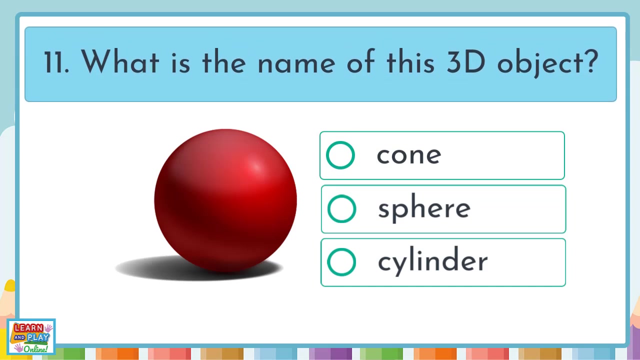 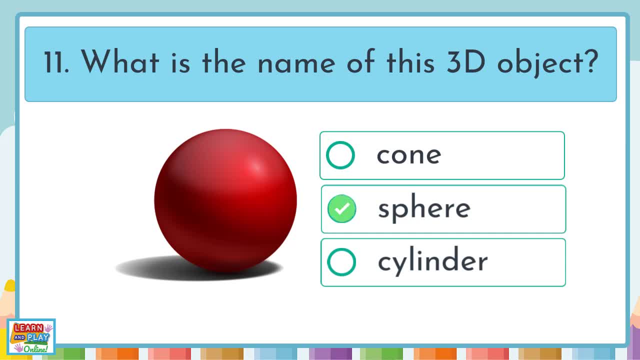 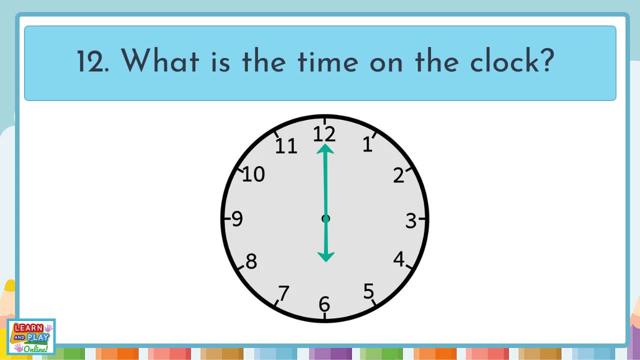 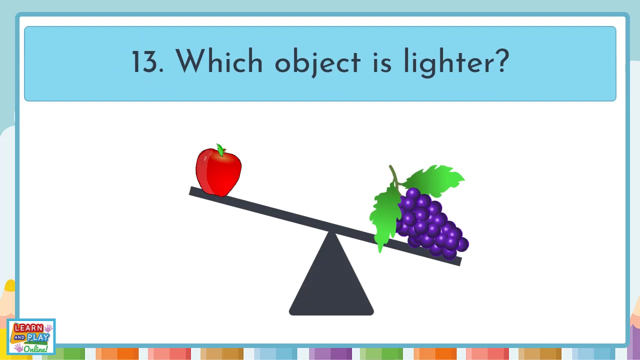 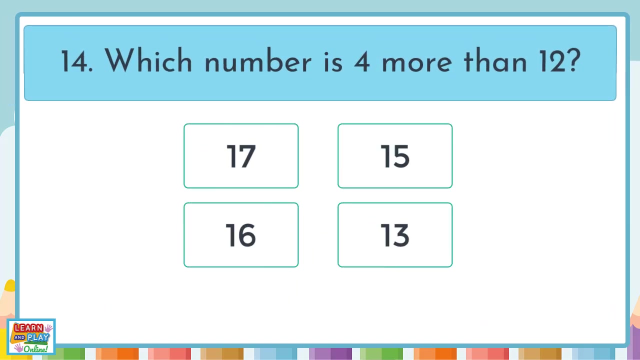 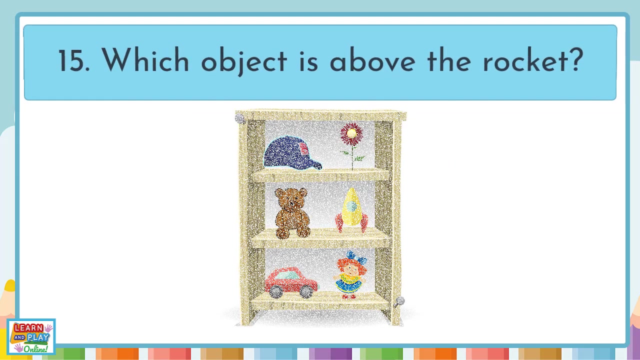 It's a sphere- Question 12.. What is the time on the clock? It's six o'clock, Question 13.. Which object is lighter? The apple, Question 14.. Which number is four more than twelve Sixteen? Question 15.. Which object is above the rocket? 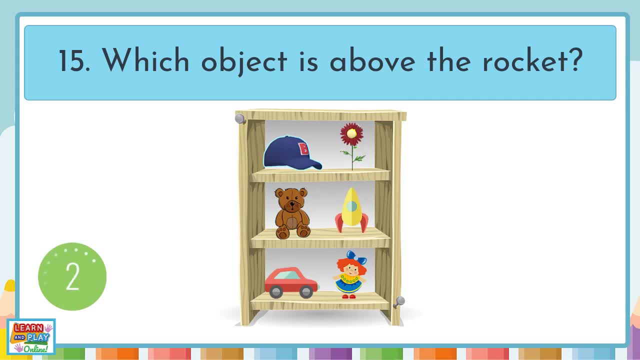 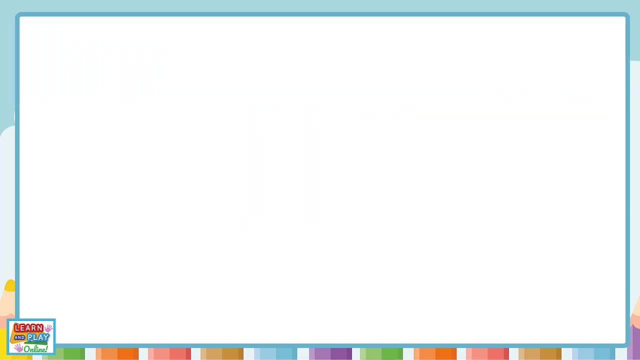 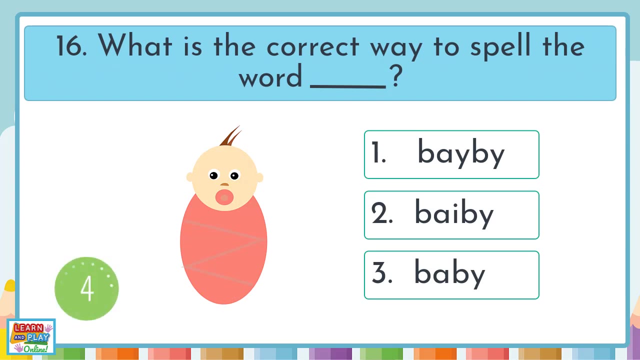 The rocket, The flower. Question 16.. What is the correct way to spell the word baby? Question 17.. Question 18.. Question 19.. Question 20.. Question 21.. Question 22.. Question 23.. Question 24.. Question 25.. Question 26.. Question 27.. Question 28.. Question 29.. Question 30. Question 31.. Question 31.. Question 32.. Question 33.. Question 34.. Question 35. Question 36.. Question 37. Question 38. Question 39. Question 40. Question 40. Question 41. Question 41. Question 42. Question 42. Question 43. Question 44. Question 44. Question 45.. Question 46.. Question 47. Question 48. Question 49. Question 50. Question 51. Question 51. Question 52. Question 52. Question 53. Question 53. Question 54. Question 54.. 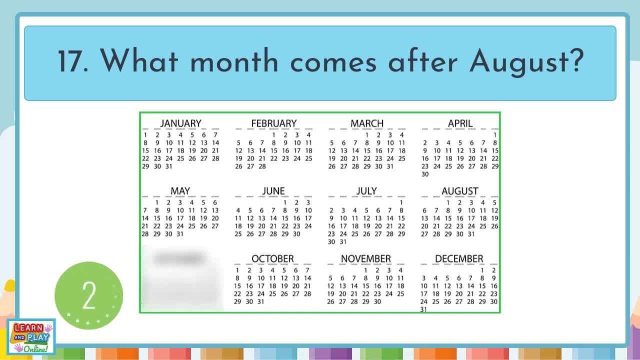 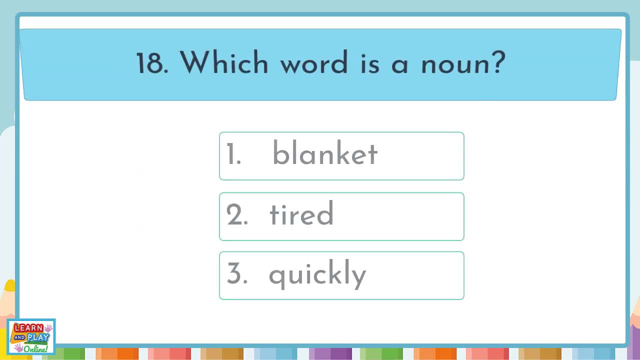 Question 55. Question 56. Question 56. Question 56. Question 57. Question 57. Question 57. Question 56.. 가 win in English. Question 18.. Which word is a noun blanket tired? you know which? 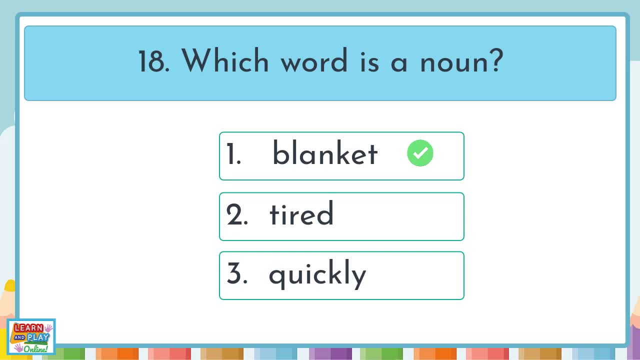 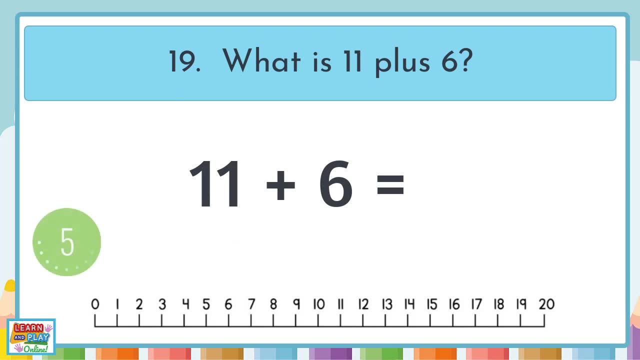 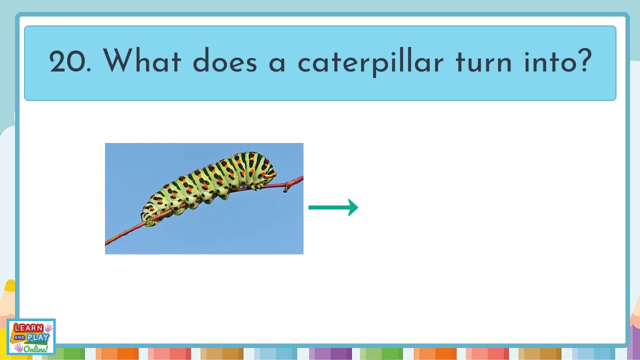 question fifty. Question ninety: Be careful. Question 9.. Question 50.. Question 자신. Question helps: Run around, Run around, Run around. And here is our last question for our quiz today: What does a caterpillar turn into?